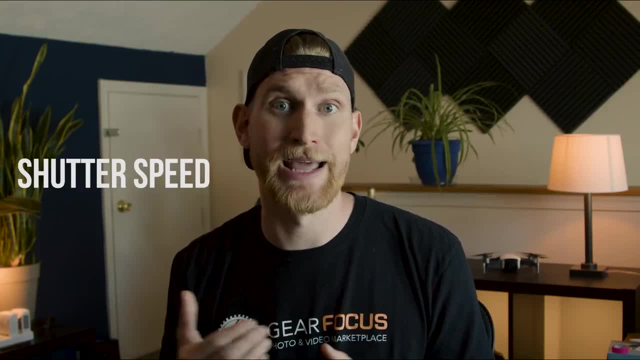 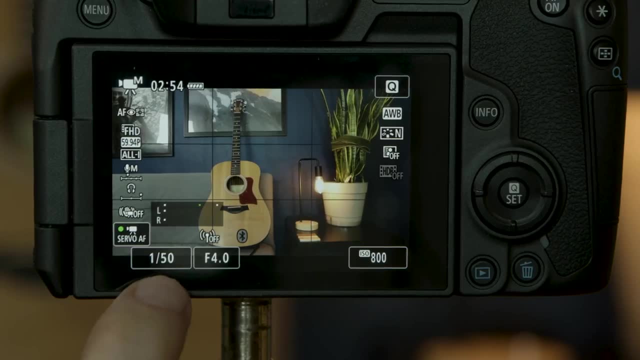 Now that's where the other two settings come into play. So next let's talk about our shutter speed. Your shutter speed measures the amount of time per second that light is going to be hitting your sensor. So when you look at your camera, that's the fraction that you're going to see next to. 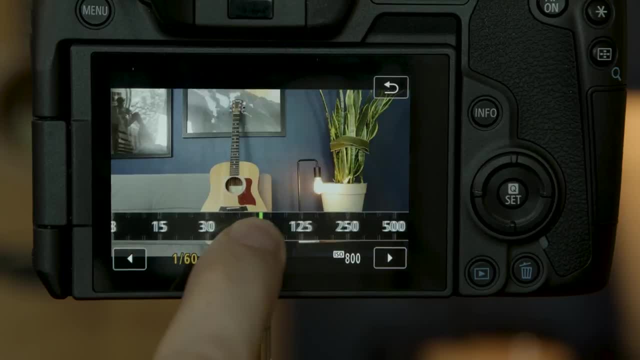 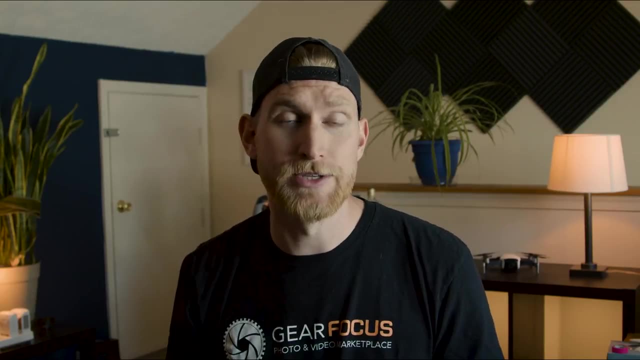 your aperture reading. Most cameras will allow you to have your shutter open for a few seconds, all the way down to a few hundredths of a second. The longer that that shutter is open, the more light we are going to get into our camera's sensor. Now there is a side effect associated. 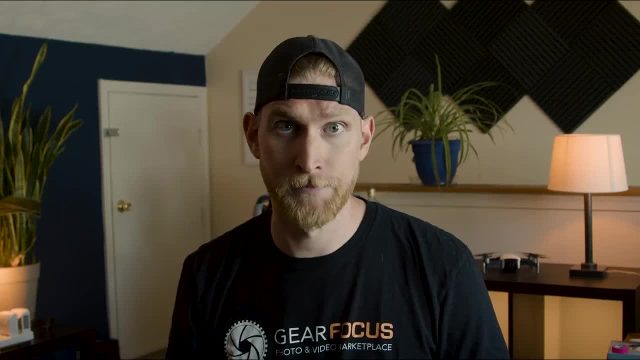 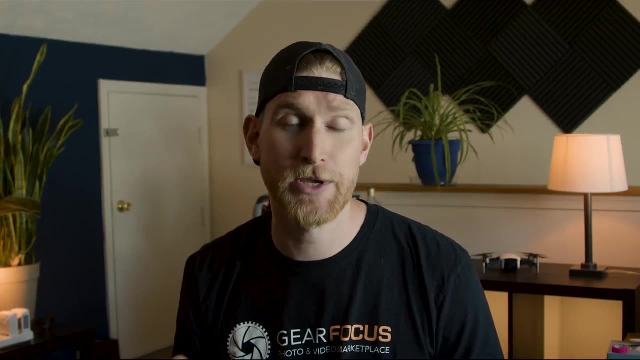 with shutter speed as well, and that is your motion blur. If your shutter is open for too long, your high motion objects in your frame are going to end up blurry, like this picture that I took at the skate park the other day. This was taken with a shutter of 1 over 200, and you can see that. 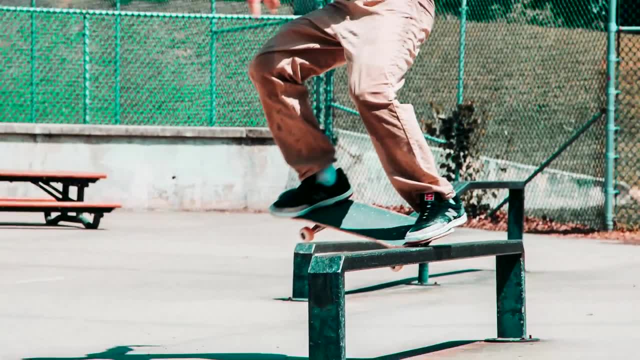 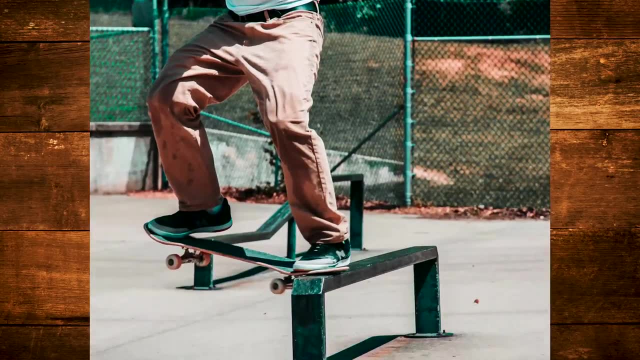 these skaters' arms are completely out of focus and they're just completely blurry. Now, if I increase my shutter speed to 1 over 800, like I did in this shot, you can see that everything in that shot is tack sharp and there is no motion blur. And the reason for that is because a fast 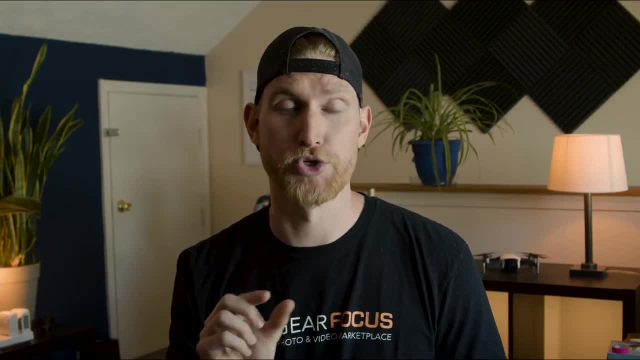 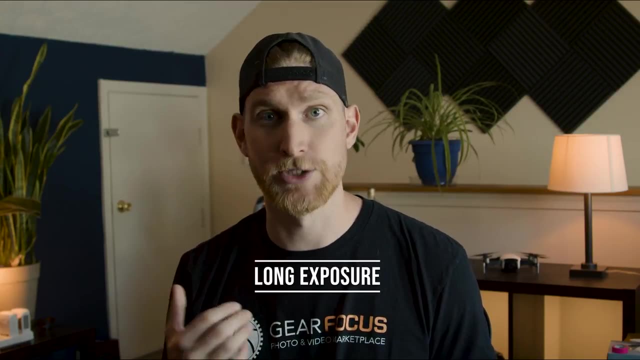 shutter means that it is taking a picture of a smaller portion of time. Now there are definitely going to be situations where you're going to want to leave your shutter open for a long period of time, and those are known as long exposures, The most common use for long exposures. 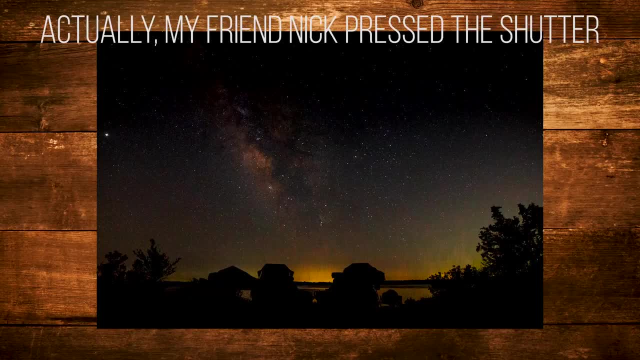 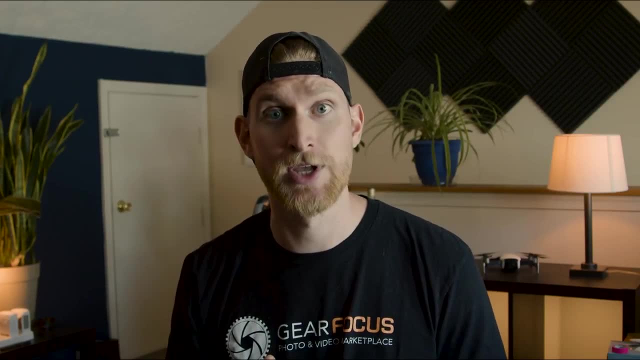 is night shots like this one that I took down in North Carolina a few weeks ago. When you have your shutter open for multiple seconds at a time, or, in this particular instance, for 30 seconds, you capture a lot more light, which means you can see the small, individual little stars. So let's talk. 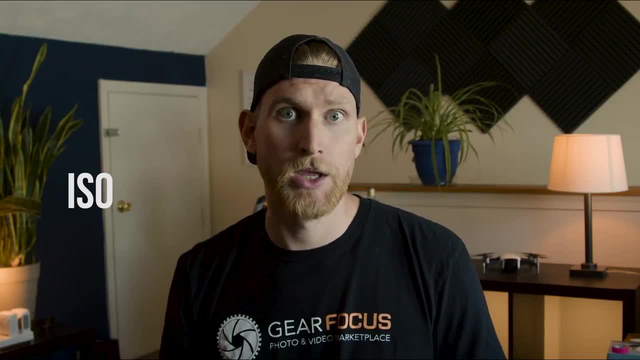 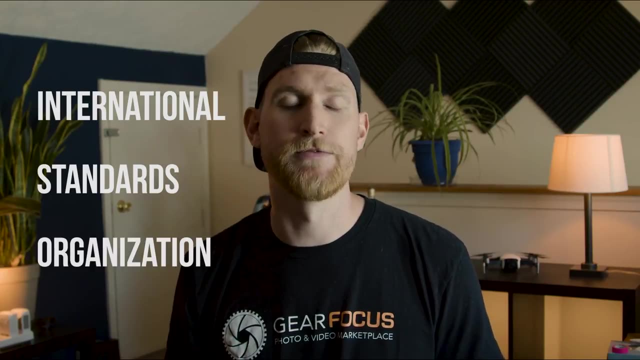 about that last main setting, which is our ISO. Now the best way to think about your ISO is kind of like a volume knob. What the ISO does is controls the amount of voltage that goes across your camera's sensor. So with a higher ISO number you're going to increase that voltage, and with a 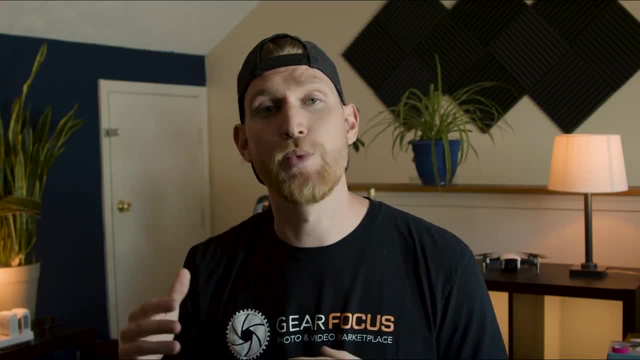 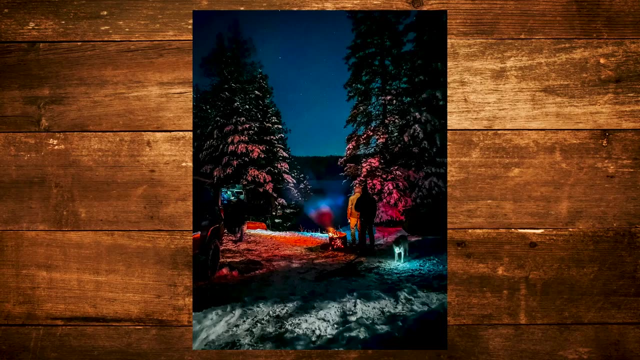 lower ISO number, you're going to decrease that voltage. Now, like with the other two settings, there is a caveat that comes into play with your ISO. The more voltage that goes across your sensor means you're going to introduce more noise into your image, which is not going to necessarily.